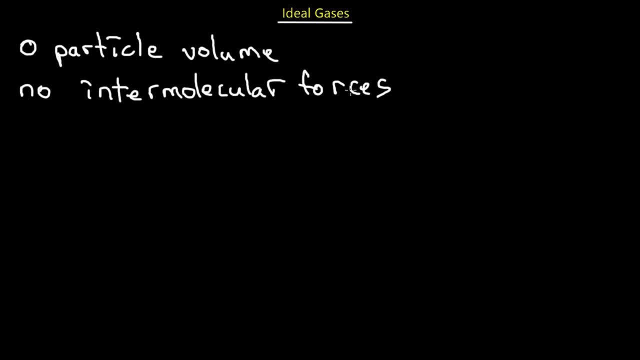 to be counted as part of the equations, because if they are counted as part of the equations, well then that's going to change everything and our ideal gas formula or ideal gas equation is simply not going to be accurate. but the only reason it does turn out to be accurate is because we assume that the gases that are involved within our equation 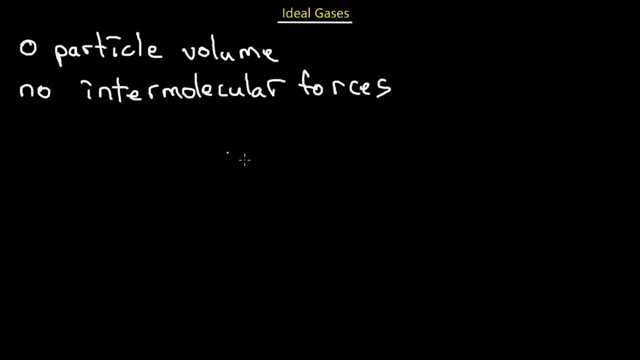 are the ones that we're calculating. They have zero particle volume and no intermolecular forces between them. Now we can confidently say that volume is dependent on two primary factors, and that is going to be temperature, measured in Kelvin, and pressure. that's typically measured in pascals or kilopascals. Now the pressure of gas. so if you're talking about 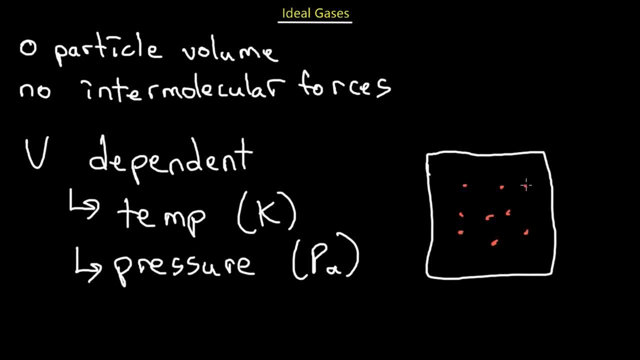 gas that is in a confined container right and you have plenty of gases in the container. the pressure of gas it where does it come from? I mean, if you have a balloon right and you're squeezing down on the balloon, it's exerting a pressure of gas. that's. 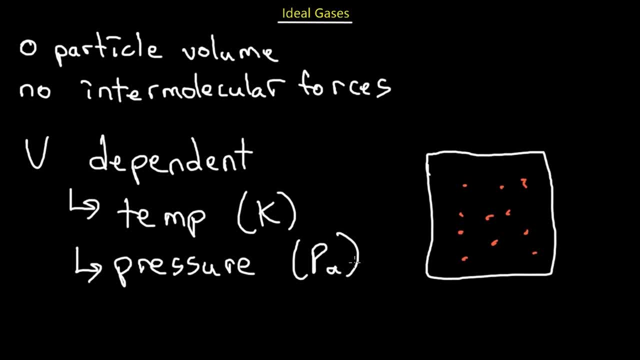 going to push the pressure against you, against your hands, as you're pushing it down, and eventually the balloon is going to pop if you keep doing that. and the reason for that is because Because it's decreasing the volume, and when you're decreasing the volume you're increasing the pressure. so they're going to have an inverse relationship between if you are decreasing pressure, you will increase volume, and vice versa. 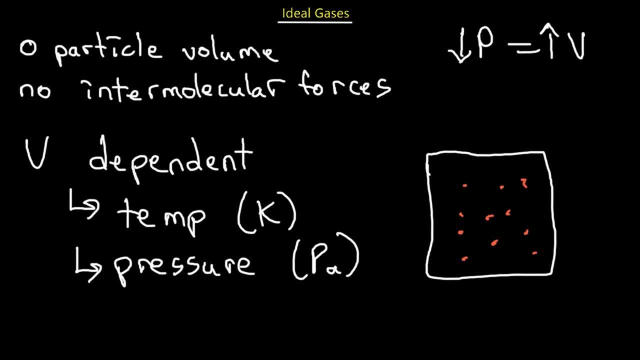 And so, in terms of containers, where this pressure come from? It just comes from the container at that point of time. in terms of gases, They're not solids, right, They're not liquids. Where does the pressure come from? Well, the pressure of gases comes from the gas molecules colliding. 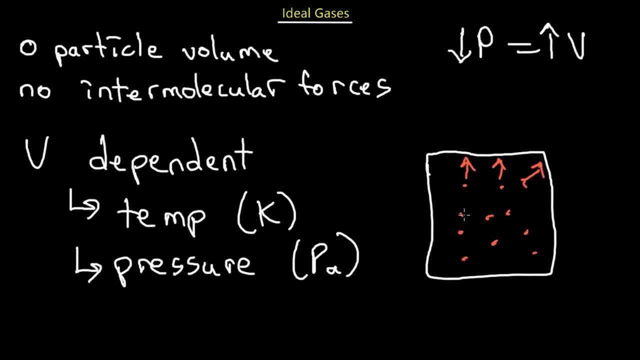 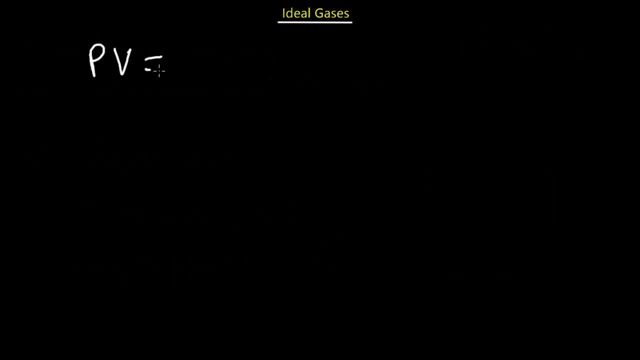 within their walls and other gas molecules within the container. That's what produces the pressure. Now, the ideal gas formula is: PV equals NRT. So here what we've got is P is of course pressure in atm atmospheres, or kilopascals, depending on which units you're. 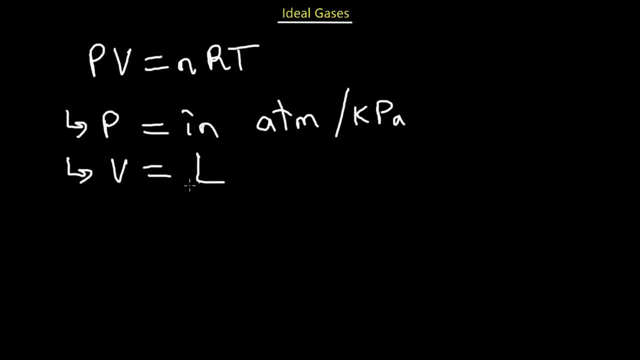 going to be using or which units are given. Volume is going to be measured in liters. We're going to have N, that is number of moles. R is going to be a constant, And so the constant measure that we're going to typically use is probably going to be a constant of N. 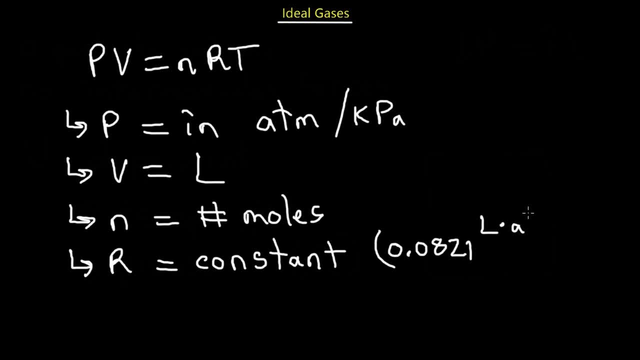 And there's also going to be 0.0821 liters atm over Kelvin times moles. So this is the typical constant that we're going to use, And a temperature will always, always, always, be measured in Kelvin. Now, if you want to know a conversion between degrees Celsius to Kelvin, 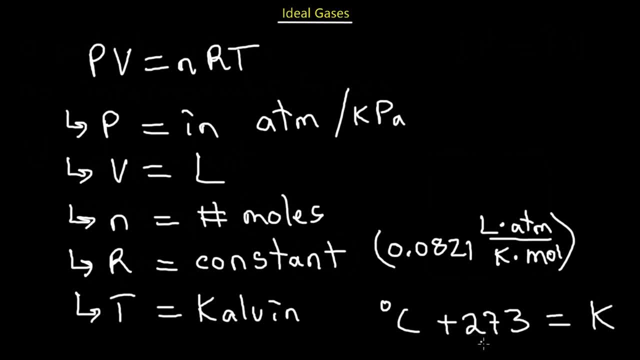 you would have to add 273 to get Kelvin. So sometimes on the IMAT you will be given degrees in Celsius and you're going to have to convert them to Kelvin by just knowing this simple conversion. Now I'm not sure how useful this is going to be for you, but something to consider is that one atmospheric pressure is going to be equal to 101.3 kilopascals. 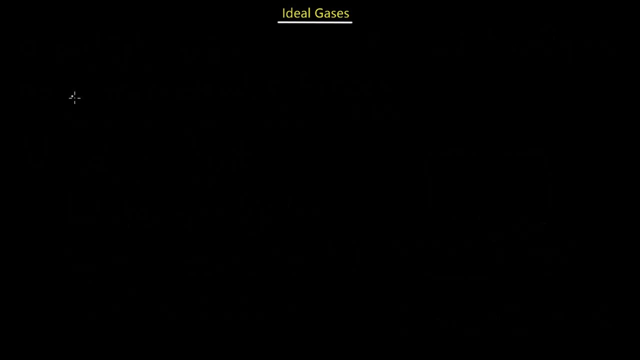 That is another unit of conversion. Now, another point of discussion here is that one mole of an ideal gas will take up 22.4 liters of volume at STP. What does STP mean? It stands for standard temperature and pressure, And what that means is a standard temperature is 0 degrees Celsius or 273 Kelvin, and standard pressure is going to be 1.. 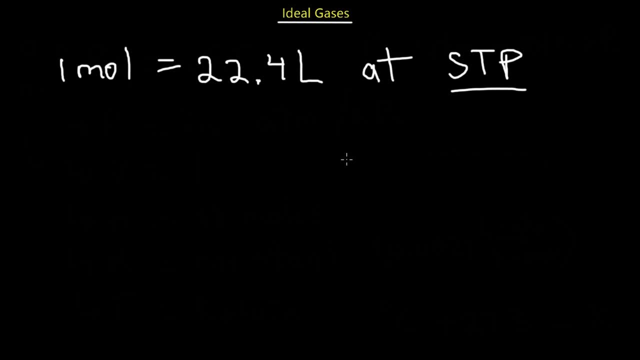 Atm or 101.3 kilopascals. So when you are given a question that states that a gas is at STP, you can make the assumption that the gas is an ideal gas and therefore you can use this sort of conversion. 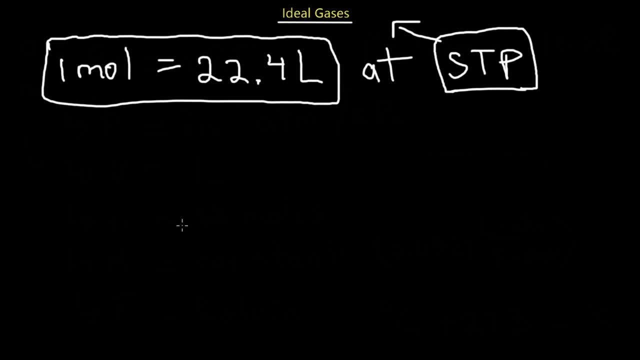 So if it's asking you for the volume that the gas takes up, then you can use the conversion from moles to liters. Or if it's asking you for the moles, then you can make the conversion from volume to liters. Or if it's asking you for the volume that the gas takes up, then you can use the conversion from moles to liters. Or if it's asking you for the volume that the gas takes up, then you can use the conversion from moles to liters. Or if it's asking you for the volume that the gas takes up, then you can use the conversion from moles to liters. 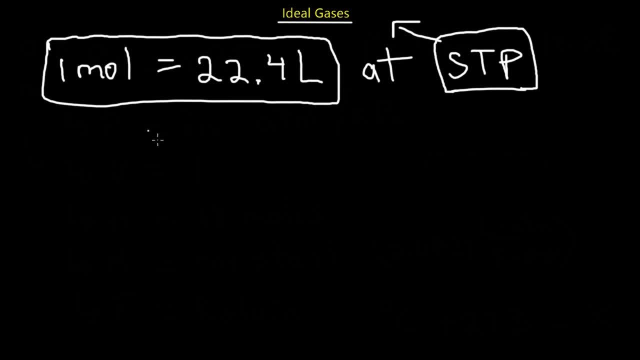 Using this same conversion, And this is something that's not given on the test, so I suggest you memorize it and you use it and practice with it before writing the IMAT. So now here we're, going to get a chance to use our PVNRT formula. 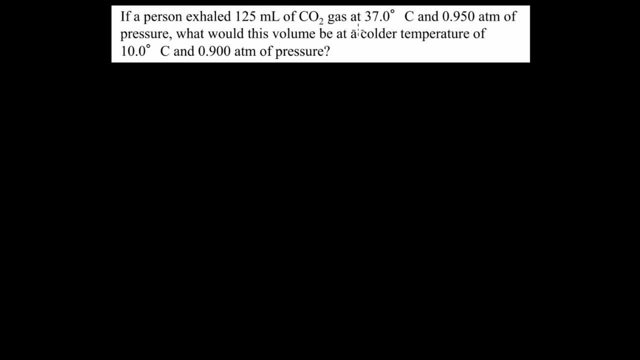 If a person exhaled 125 milliliters of carbon dioxide gas at 37 degrees Celsius and 0.95 atm of pressure, what would this volume be? What would this volume be at a colder temperature of 10 degrees Celsius and 0.9 atm of pressure? 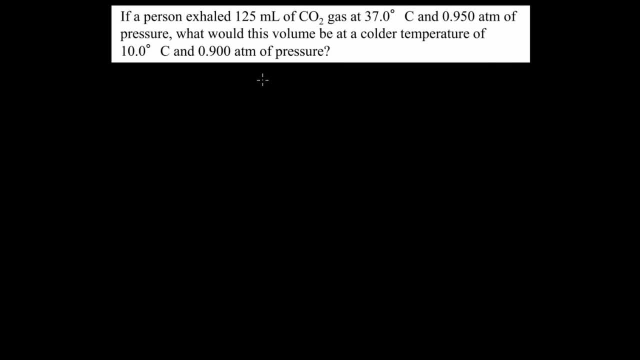 So what I gather from here is we have two situations. The first situation gives us everything except for moles, except for N, And the second situation gives us just the pressure and the temperature. So what we're going to have to do is basically find our number of moles, so that then we can find the volume, the second volume that is being measured. 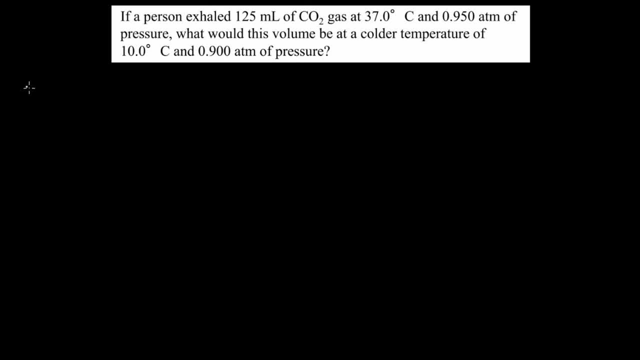 So we're going to have To do PVNRT twice. So first of all, I'm going to convert the 37 degrees Celsius into Kelvin. That will be 310 Kelvin. That is the temperature that we begin with. So the formula is: PV equals NRT. 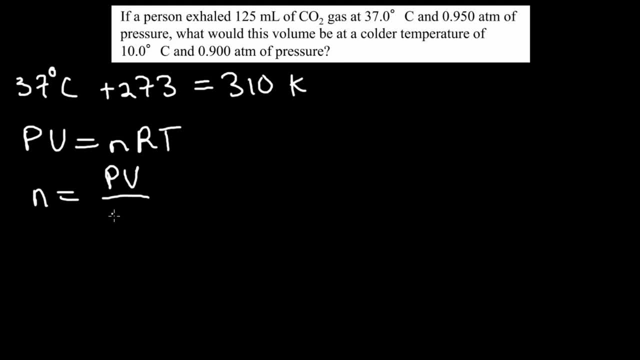 Now, in order to isolate for the moles, N is going to be PV over RT And I'm not going to go over the math here right now and how I got there. That's going to be something that will be dealt with them with the math unit. 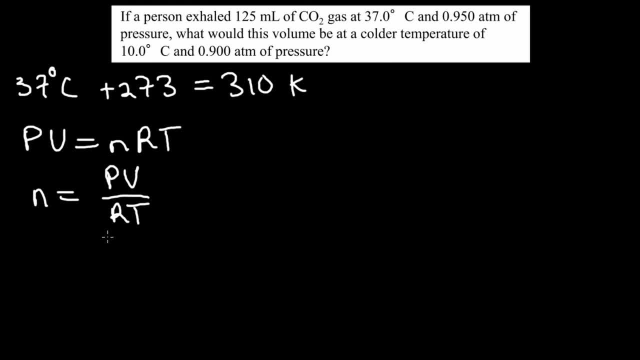 So if you cannot do this basic conversion, I suggest you drop chemistry right now and you go do a little bit of basic algebra. So now we are going to substitute all of our variables in for the first situation. So our pressure is 0.950 atm. 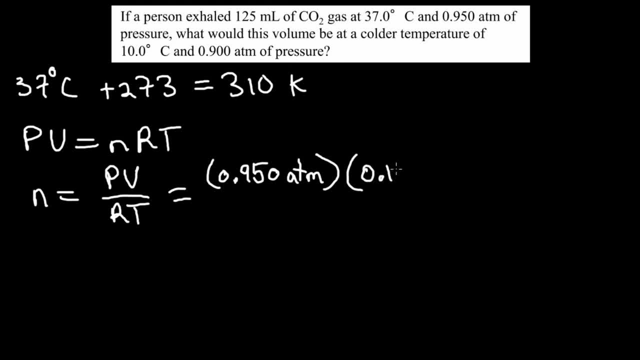 That will be multiplied by the volume. I'm going to convert the volume into liters, So there'll be 0.12. 5 liters. Also, you're going to need to learn some basic unit conversions like milliliters to liters and degrees Celsius to Kelvin, possibly atmospheres to kilopascals. 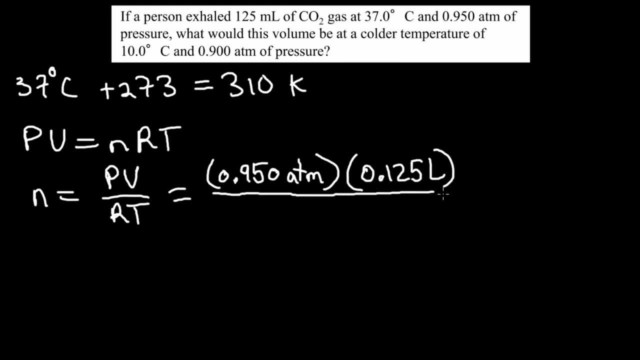 You're going to have to learn some basic unit conversions along the way. That will be over R, So our constant is going to be 0.0821 liters times atm over Kelvin, And that will be multiplied by 310 Kelvin in terms of temperature. 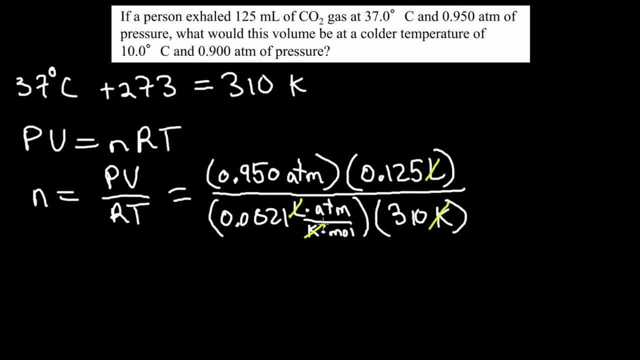 So now I can cancel our units. Kelvin will cancel with Kelvin, Liters with liters, Atmospheres with atmospheres. And now, because this is in the denominator of the denominator, we are going to get our units as moles. So let's do the calculation here. 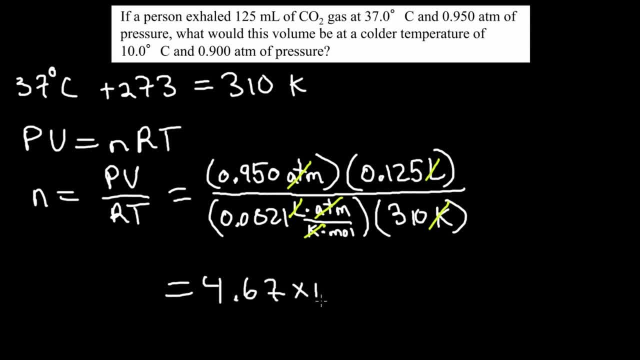 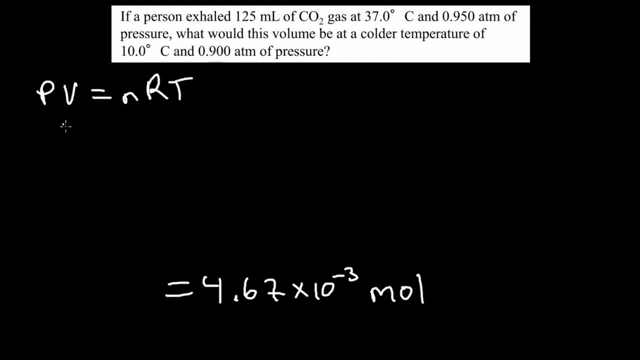 So our answer is going to be 4.67 times 10 to the negative 3 moles, And I would suggest you also learn how to convert from decimals to scientific notation for the chemistry unit as well. Now I'm going to rearrange my formula to find the new volume with the new temperature. 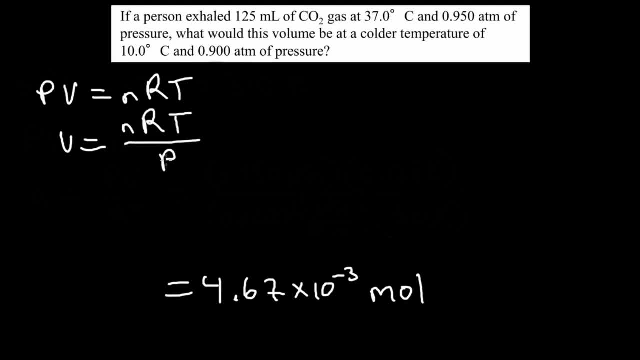 So volume will equal nRT over p. This will now equal to 4.67 times 10 to the negative 3 moles that we calculated within our previous equation. R is going to stay the same: 0.0821.. 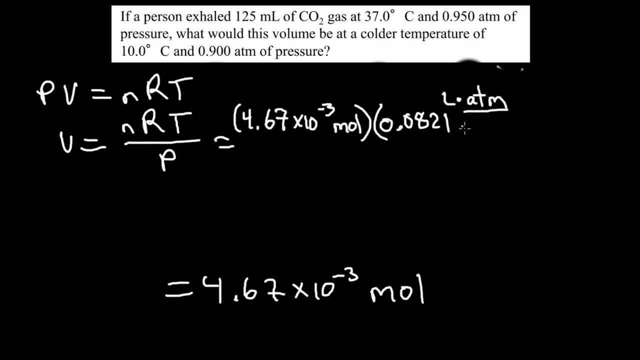 Remember, it's a constant, So it remains the same. Our temperature is now going to be 10 degrees Celsius, So 10 degrees plus 273 is going to be 283 Kelvin, All over new pressure of 0.900 atm. Now let's do the cancellations. 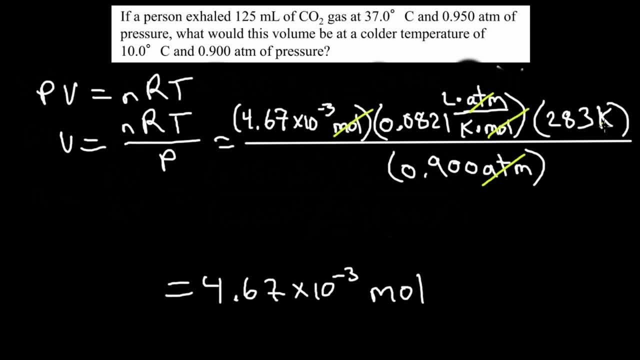 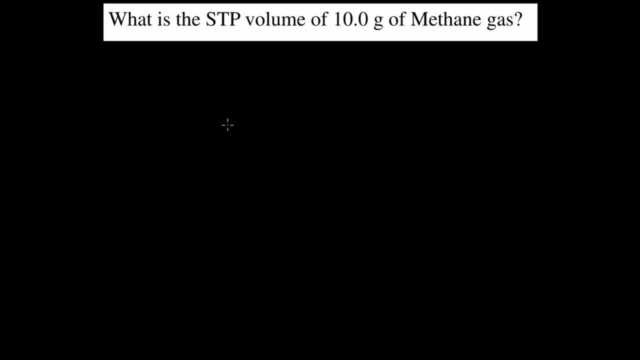 Atmospheres cancel with atmospheres, Our moles will cancel with moles, Kelvin with Kelvin, And we're left with liters. on the numerator of the numerator, The answer is 0.12 liters. Next is going to be a little bit of stoichiometry. 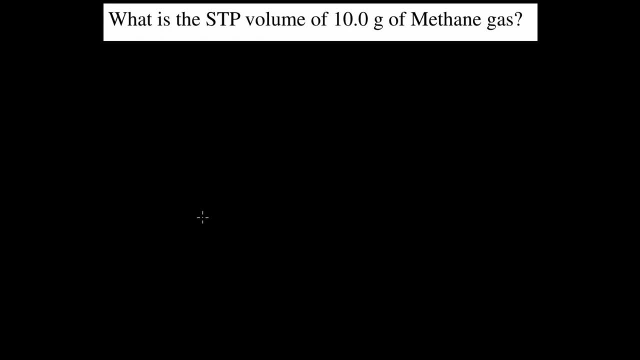 And we're going to get into stoichiometry a little bit later in chemistry, But for now, since this involves the ideal gases and the ideal gas equation, I figured I might as well bring it up. So the question is: what is the STP volume of 10 grams of methane gas? 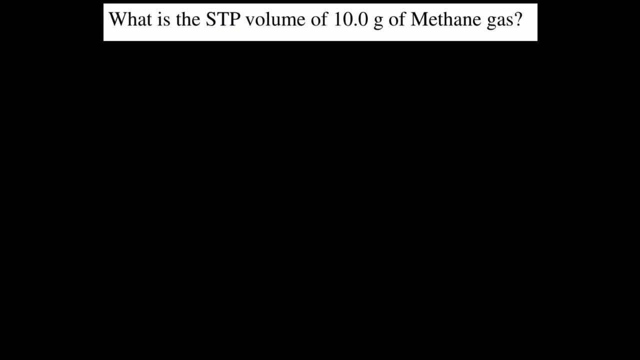 Again. I've mentioned this previously. STP stands for standard temperature and pressure, which indicates to me that it is talking about an ideal gas. Therefore, I can use the conversion of 1 mole to the 22.4 liters of volume. 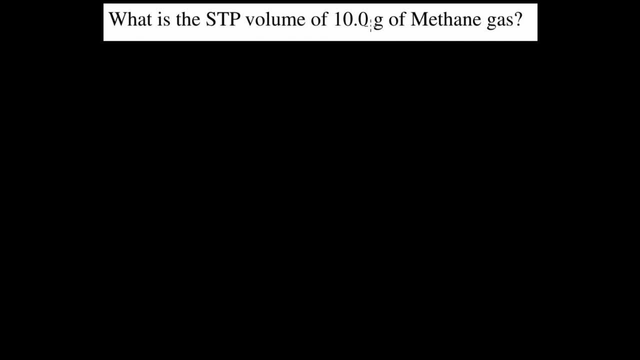 It's asking for the volume. So again, what we're going to have to do is take 10 grams of methane Gas and turn it into moles and then turn it into our liters for the volume. So first always start with what's given. 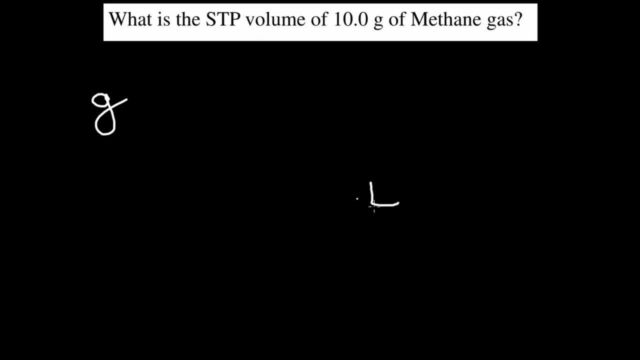 I'm given grams and I need to get to liters of volume. I cannot go there directly, So what I'm going to have to do is convert it to moles, because I'm going to know what the molar mass of methane is by looking at the periodic table. 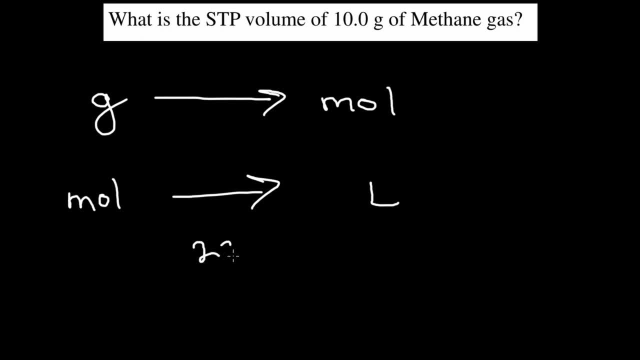 And from moles. I'm going to be able to go into liters Using that 22.4 conversion that we have at STP. So let's begin. We've got 10.0 grams of methane gas. Now the formula for methane gas. 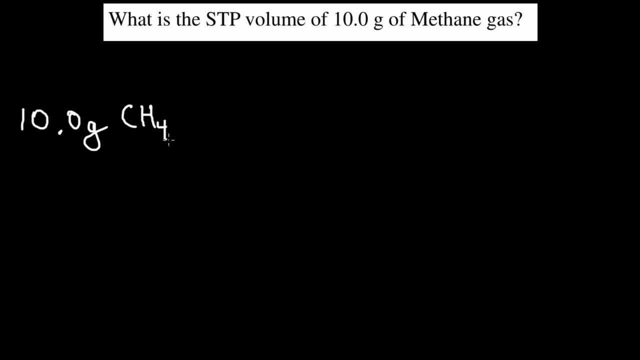 and this is something we're going to learn in organic chemistry- that is, CH4.. So now what we're going to have to do is use the periodic table to add up the molar mass of carbon and the molar masses of four hydrogens together. 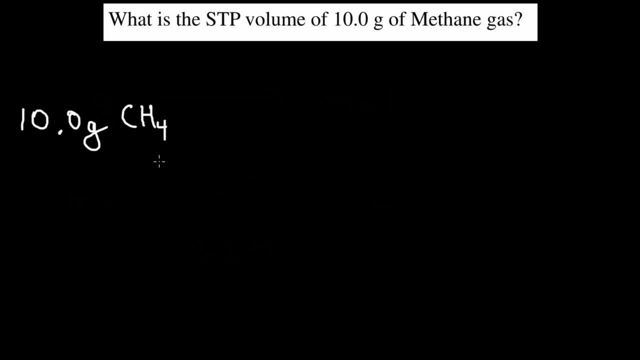 So carbon, the molar mass is 12.011.. We're going to add 1.008, the molar mass of hydrogen multiplied by four, And our molar mass is going to be 16.043 grams per mole. So when I multiply, 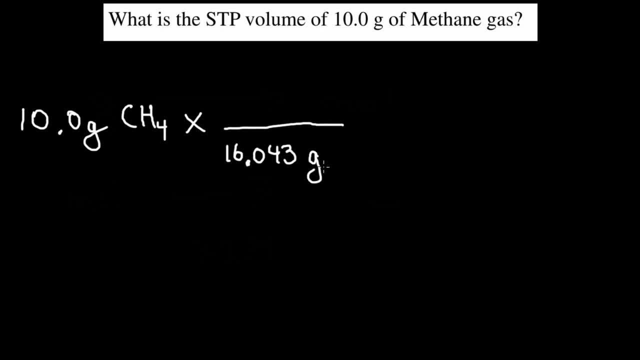 I'm going to have the grams in the denominator in order to cancel with the grams that were given, And I'm going to convert that into moles. One mole of CH4.. This is molar mass. This is the reason I can convert that. 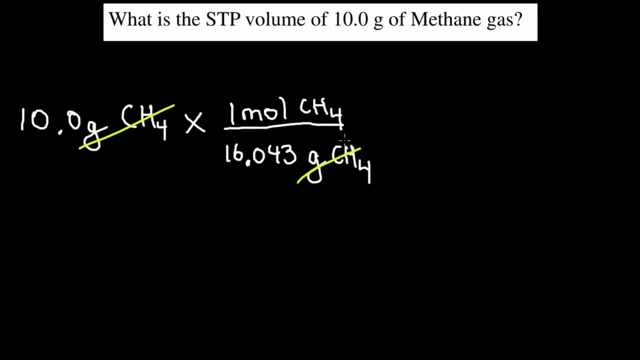 Now the grams will cancel. with the grams We're left with moles. Great, But I need volume. So I'm going to convert moles to volume by doing the conversion of one mole of an ideal gas, That is CH4 gas, into 22.4 liters.